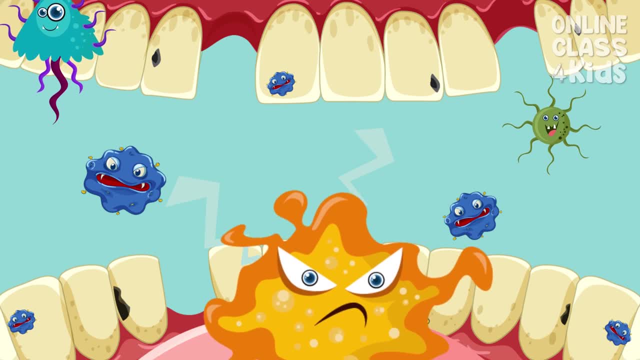 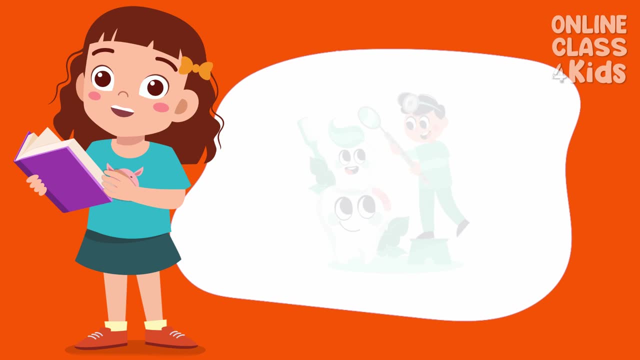 Brushing Teeth. Did you know that our mouth is one One of the dirtiest parts of our body? Yikes right. That is why you should always brush your teeth before and after eating. We can only have two sets of teeth, so we really need to take care of them. 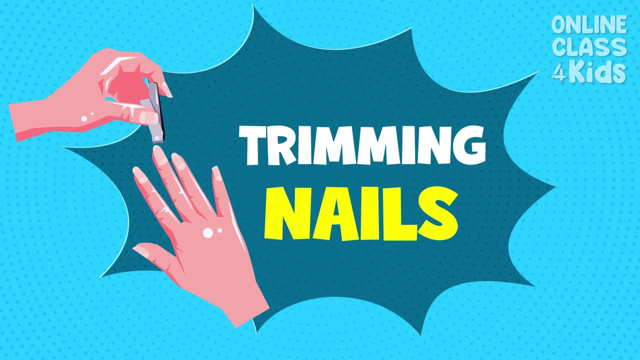 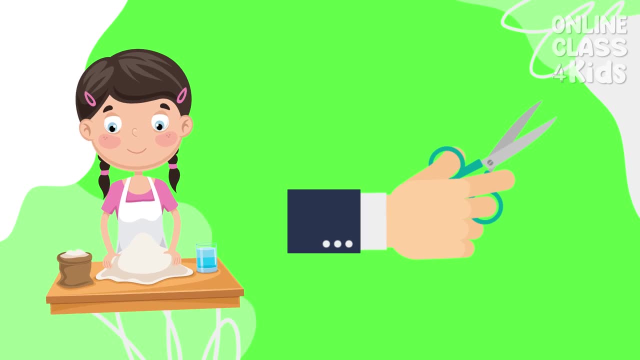 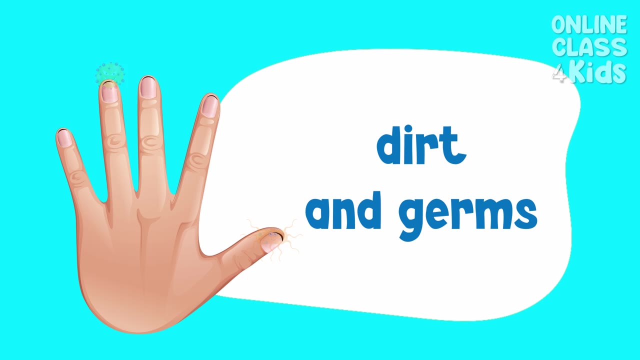 And lastly, trimming our nails. As part of our hands, the nails also get in touch with a lot of things, including dirty ones. A lot of dirt and germs can get stuck in the nail when our nails are long, so we have to trim them often. 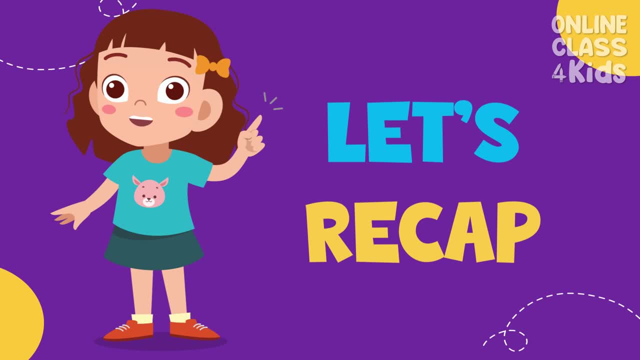 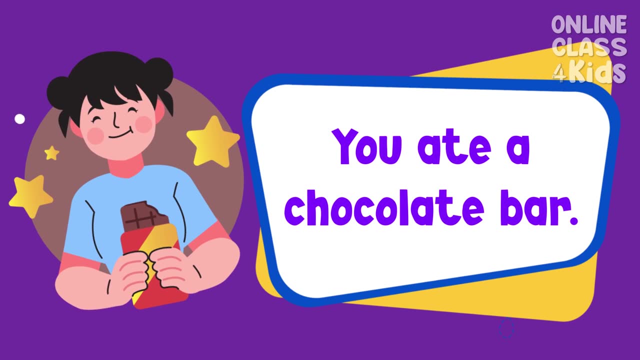 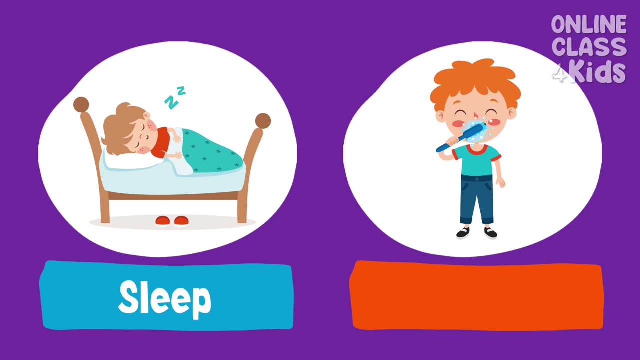 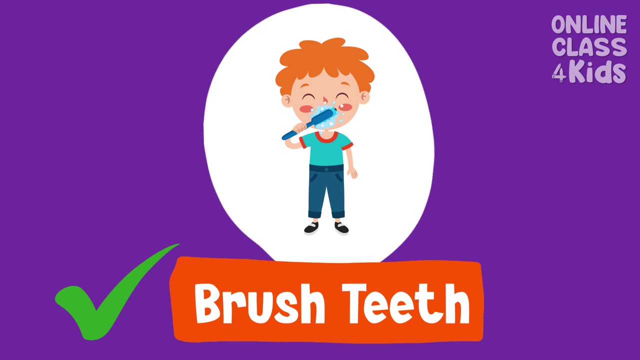 Let's have you recap. shall we Choose the correct answer from the two choices? You just ate a chocolate bar. Do you sleep or brush your teeth? That's right, You brush your teeth. We need to brush your teeth to keep it healthy and clean. 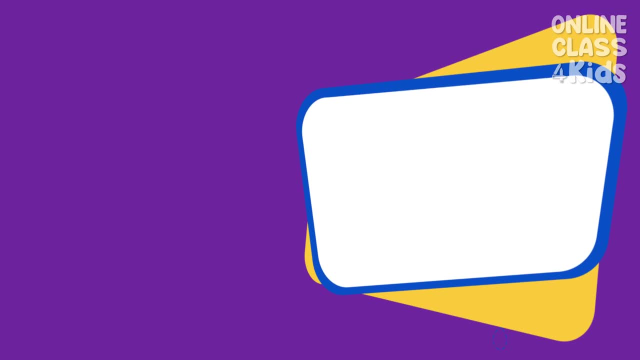 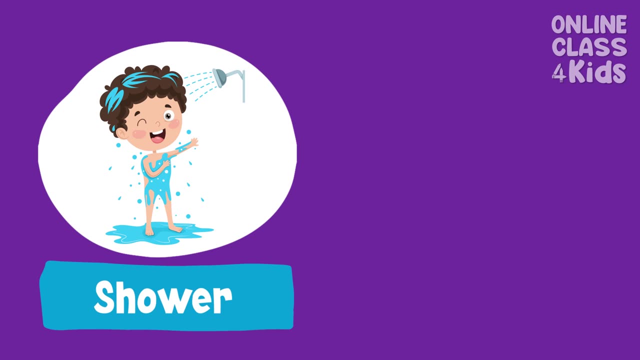 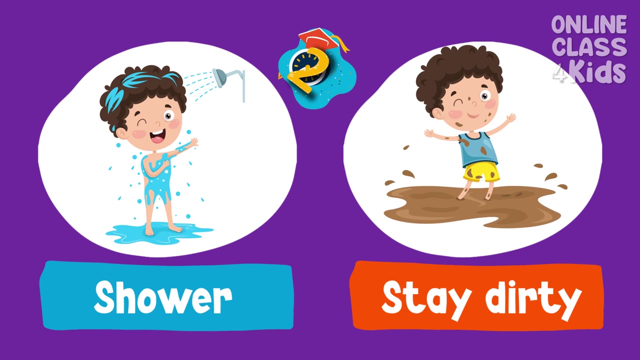 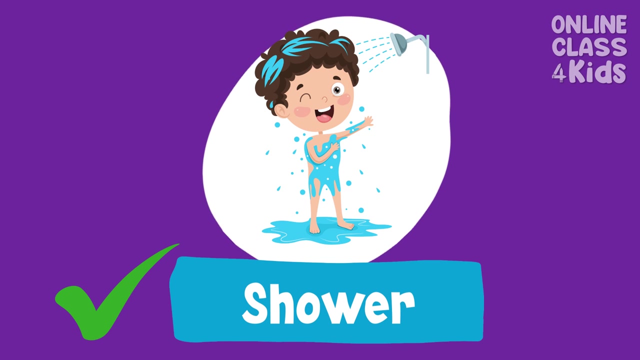 Very good, You went home dirty after playing hide-and-seek outside. Should you shower or stay dirty? That's right, You take a shower or a bath to clean out all the dirt and germs on your body. Very good, You have a habit of biting your nails. 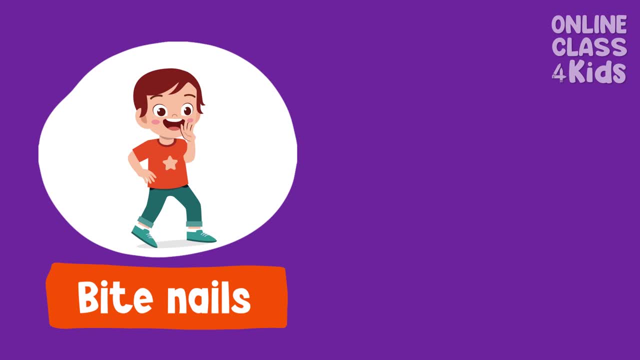 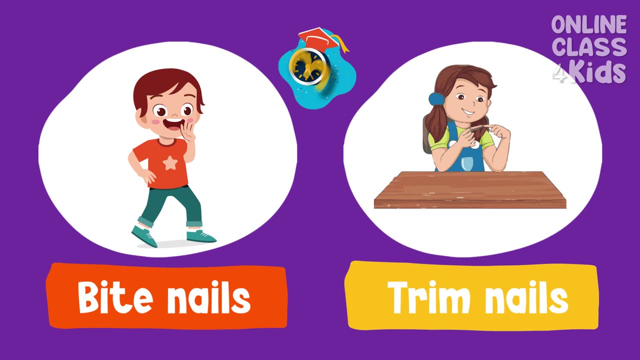 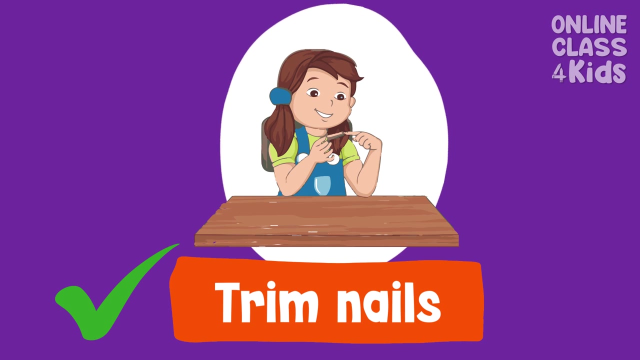 Your nails are full of dirt. You have a habit of biting your nails. Your nails are full of dirt. Should you bite your nails or trim your nails? That's right. You should cut your nails so that no germs can get stuck under your nails.